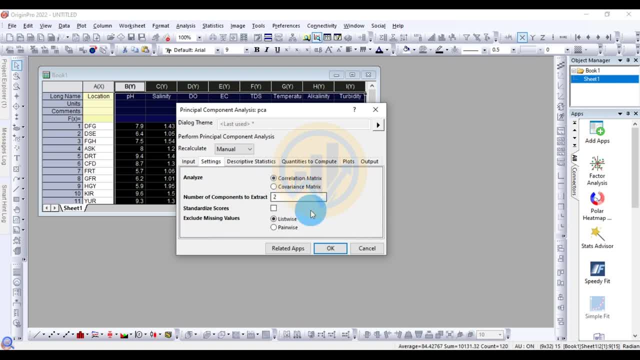 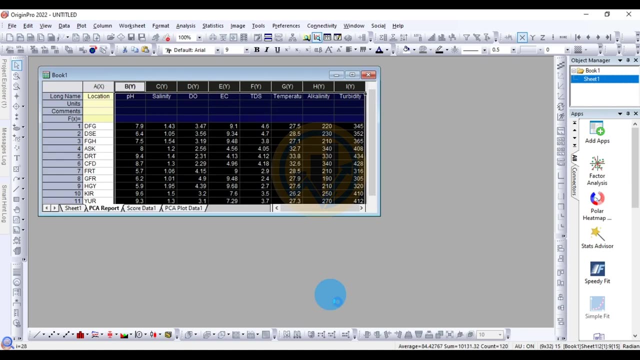 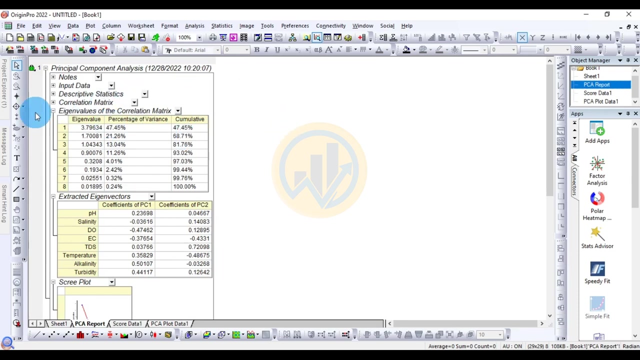 first one for the setting menu. Okay, the next go to for the hyung panel. the first go to for the manque section, then go to options and then I'll go. next go to the CI settings of the system. Okay, now we're ready for theему- an analysis for this. The first one for the 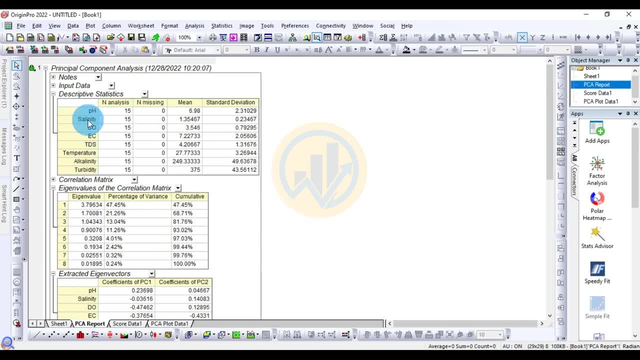 description: intelligence uniform to audit the system. after this, Let's talk about in the same way today for a driver初 epidemic test last nine week. okay, in addition to the Mori ciate, given data, the number of code. YOU began processing one copy before seeing. 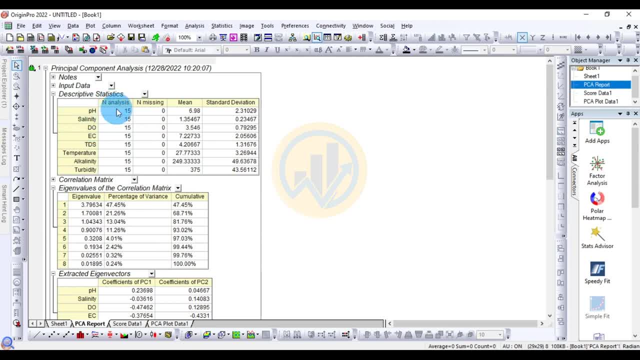 it into code experience threats. We create two and the same information class晚上. first one for the N and it says total number of sample: 15. then missing the value for the zero, the mean value for the pH, to the terminity, the P hour is. 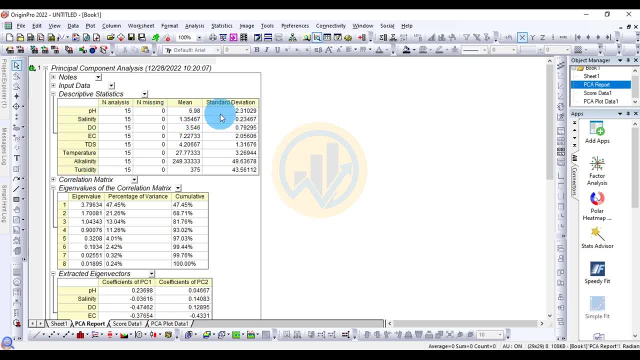 the pH value six point nine, eight under the standard deviation value two point three, one and also the same for the salinity and the devo easy, DDS and the temperature, alkalinity and the terminity, also the mean value three hundred and seventy five under standard deviation only for forty four point fifty six, the 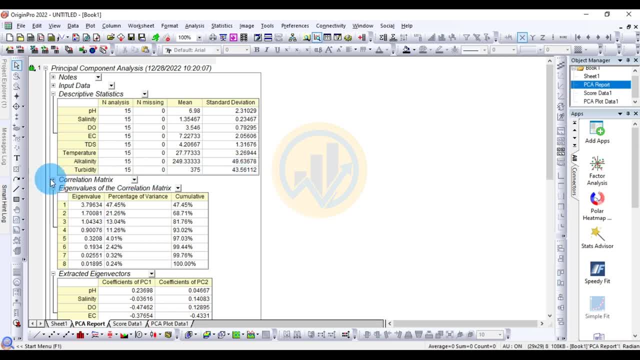 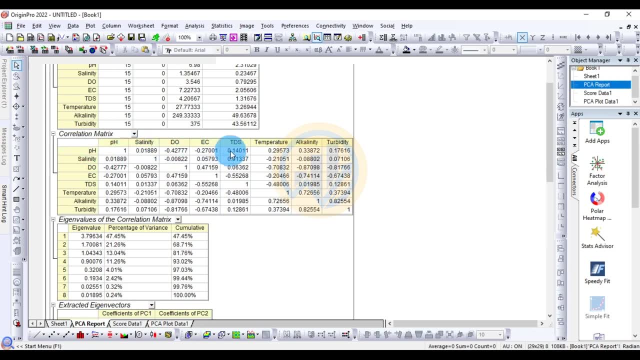 next one for the table, the correlation matrix. the correlation matrix for the pH to pH D, salinity, salinity and pH devo, pH easy, pH, DDS, pH temperature and the pH al alkalinity, pH in the terminal. so the correlation for the matrix, then biggest salinity the positive correlator and the pH devo is a negative. 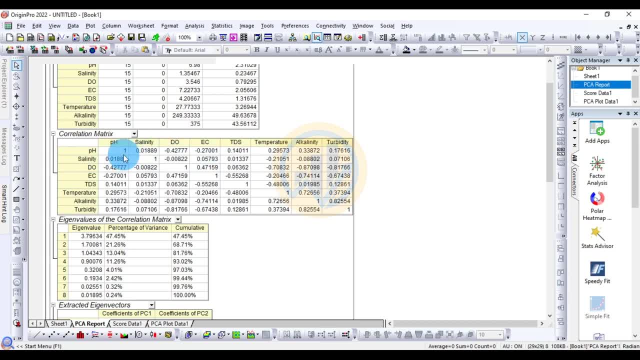 correlator, the pH is easy, also negative value, then PC, DDS, all the positive correlation, zero point one, four, and the pH term temperature, also positive correlation, the zero point two, nine, and then pH, the alkalinity also the positive, zero point thirty three, pH and determinants of positive zero point one, seventy six. the next one table for the. 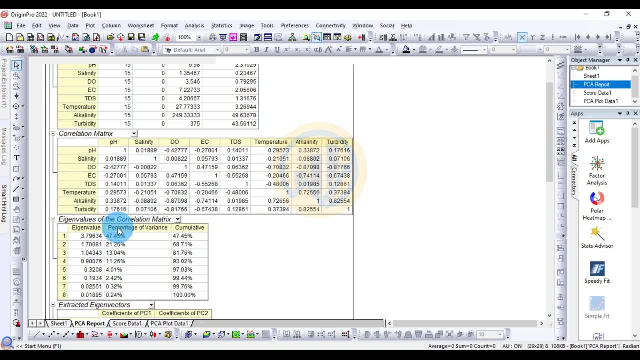 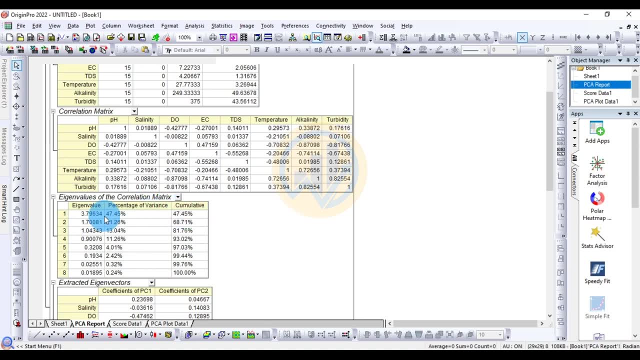 eigen value for the correlation matrix, the first one for the eight component. the eigen value and the percentage of variations and cumulative values. the first value for three point seven nine. the percentage of value for forty, seven point the forty five. the highest value of the variation, the cumulative. 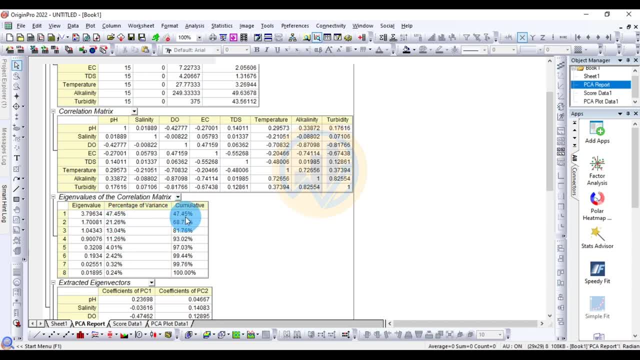 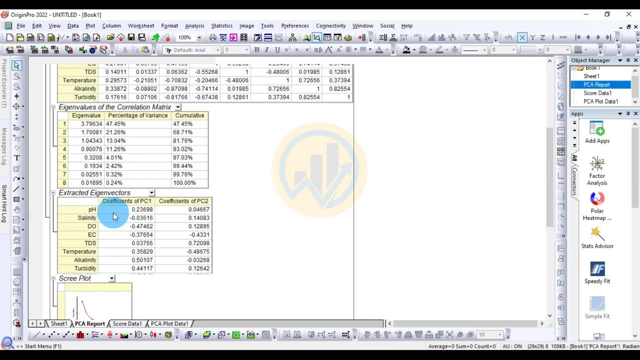 value, the forty seven point, the forty five, the eight, eigen value: the next one table for the exact eigen eigenator. then pH, the coefficient PC, PC one value on the coefficient PC two value. the pH pH value zero, point twenty three. the PC two value zero, point forty six. the next, salinity minus zero: point three, six. then PC two value zero. 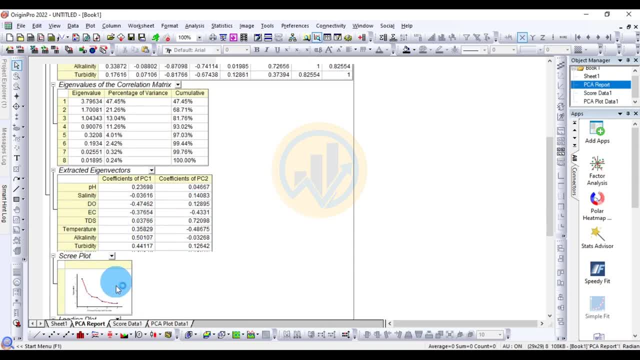 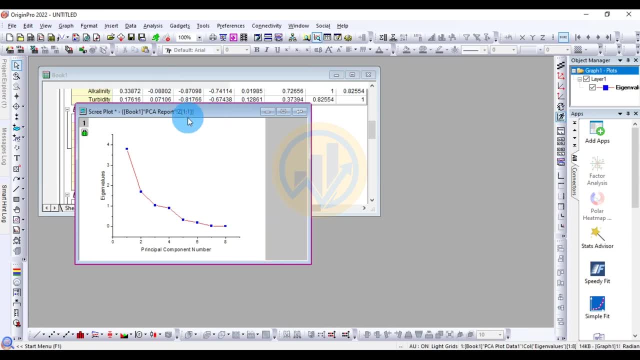 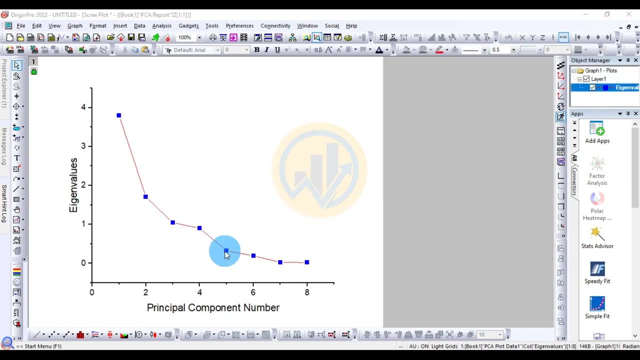 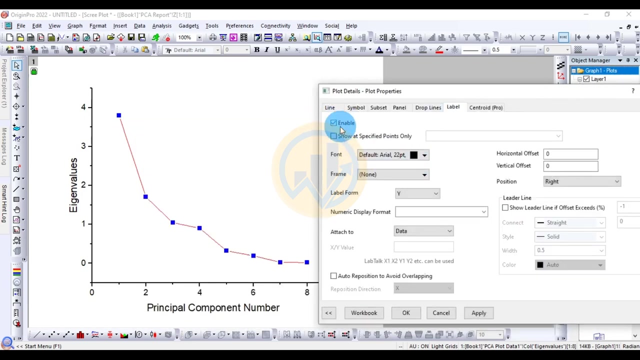 point one four. the next one for the square plot. the square plot: value for the compared to eigen value. the double click the square plot open the new tab for the square plot. okay. double click for the value dot- open the new tab. then enter the label. okay, double click for the value dot- open the new tab. then enter the label. 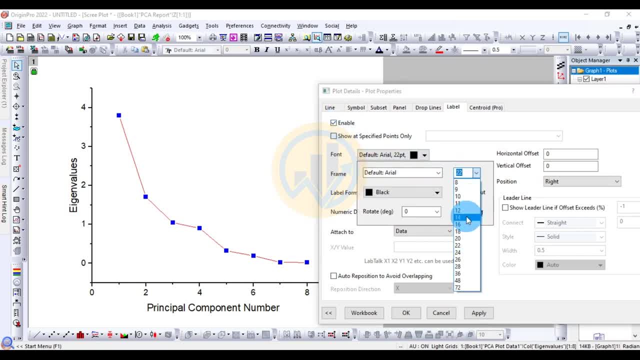 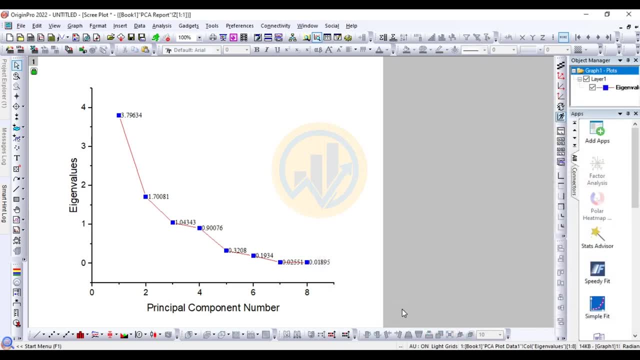 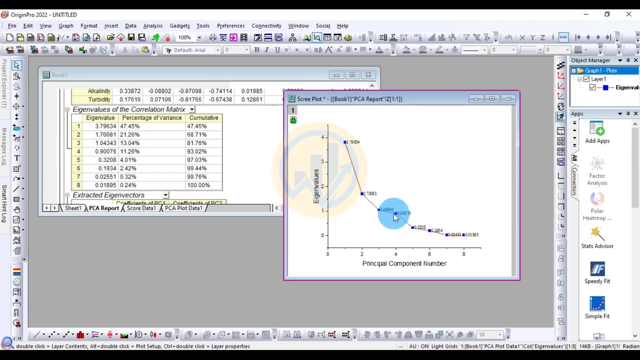 okay, double click for the value dot. open the new tab. then enter the label. then enter the value dot. open the new tab. then enter the label. then enter the label. then enable the label checkbox. the change change for the checkbox. the change change for the font size: 14 to change font for the time. 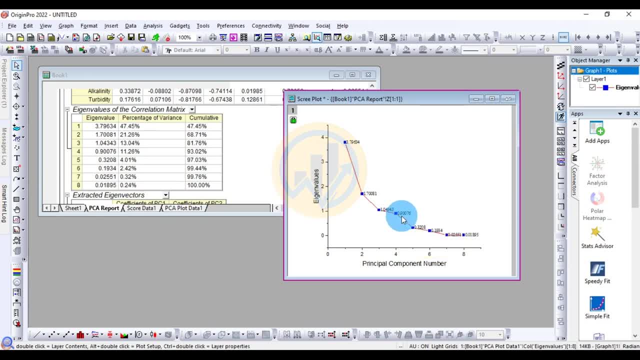 Roman. then click a plate. okay, this is a scattered plot. 1, the code type, the fourth code, the points. then cumulative value for the fourth point, 93 point for the 0 to this value to mention for the eigenvalue for the correlation matrix. okay, the next one for the 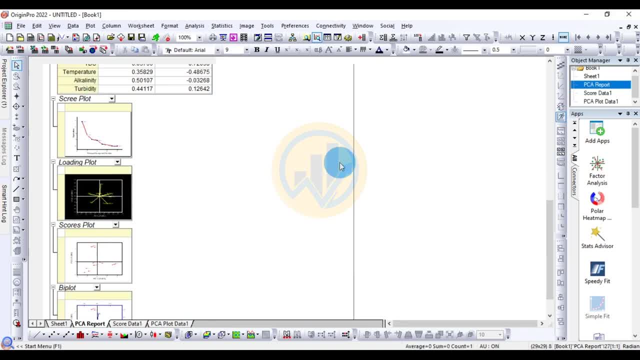 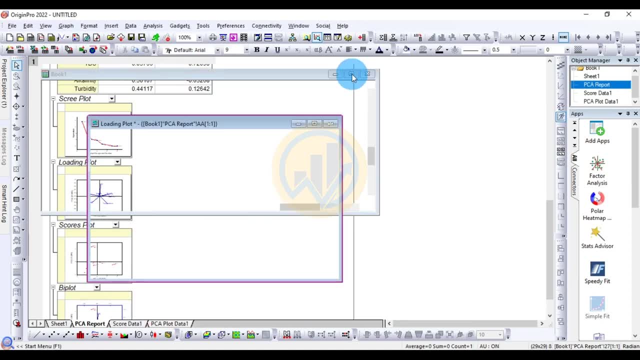 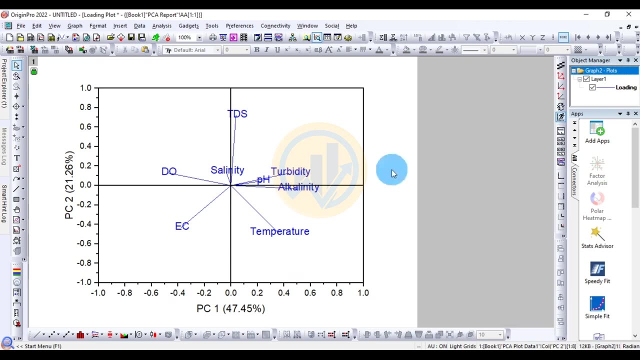 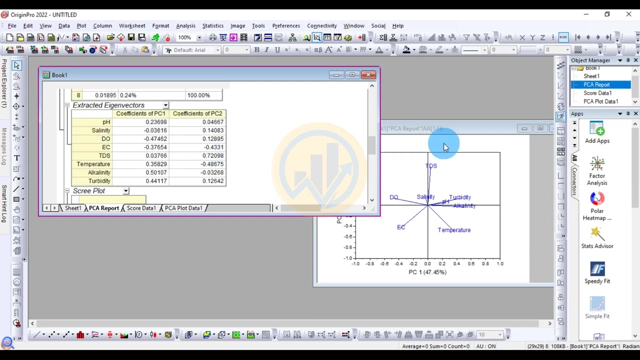 the loading plot. double key for the loading plot. okay, open the new tab. this is a loading plot for the water parameter and the positive, negative, the value, then loading that, also the mention for the, the eigenvalues, the positive, negative. the peak is also the positive for the pc1 value and the. 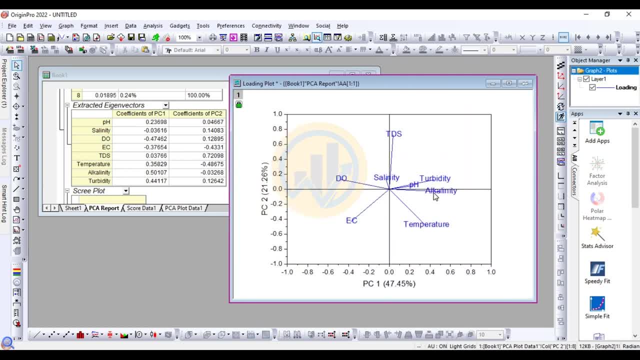 pc2 value. okay, the peak is the positive one, the principal compound for the 0.23 and the pc2 value for the 0.04, and also the minus, the salinity. the salinity is a, the pc1 value for the negative, the 0.036, and the positive for the pc2- 0.114, and also the devo. the devo also the negative for the. 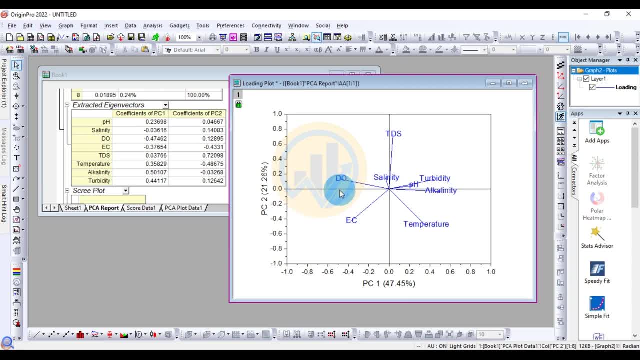 pc10 minus 0.47 and the also the negative value for the pc2, the zero point. sorry, positive for the, the def of the pc2, the 0.12, the ec also, the is also the pc1, pc2 also the negative value and the dds also dds also the positive value for the pc1 under the pc2 temperature, the pc1. 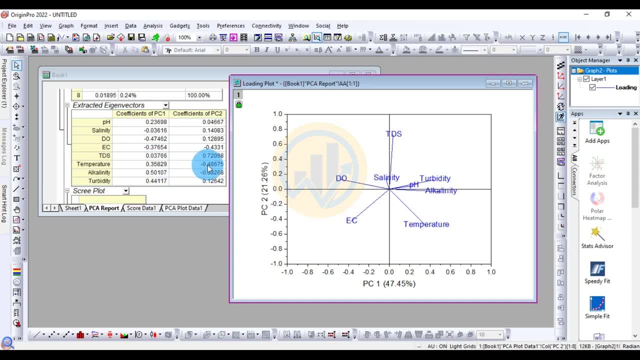 the negative positive value and the pc2 is a negative value. temperature, the next one with alkalinity: the pc1 is a positive value, alkalinity is a 0.05. the negative find, the 0.0, 3.2, the negative value and also terminity: terminity of the PC on the. 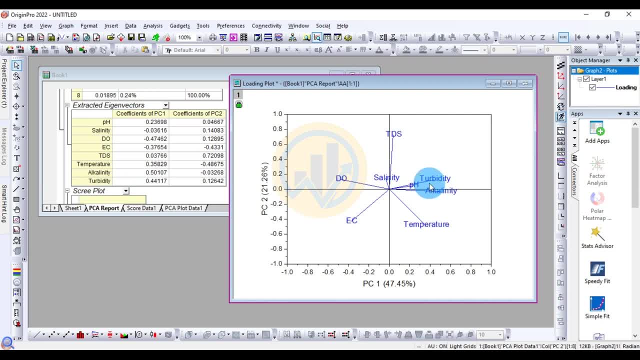 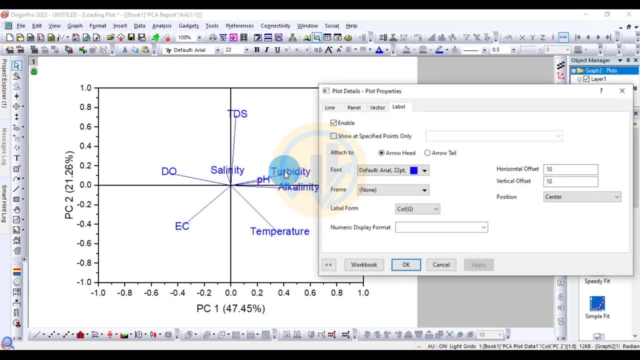 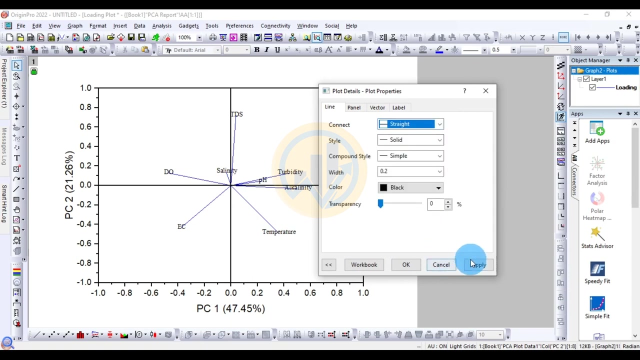 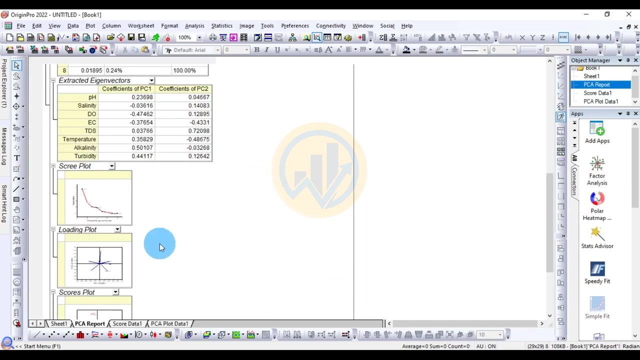 positive 0.44 and also PC2. also the positive 0.12 value. okay, the change for the WP for the water parameter and change the label for the font size, then 14, the change for the time. Roman change color the black. okay, okay, then I played the line on. so the color change for the. okay, the next one. 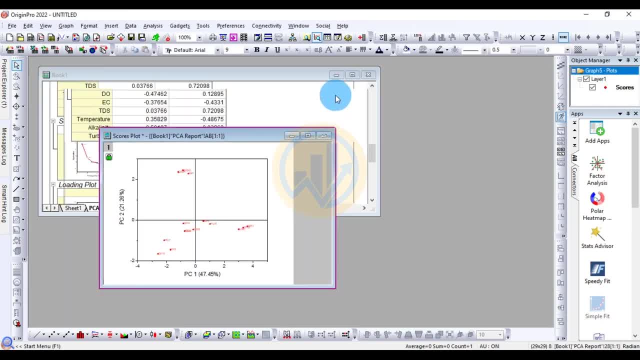 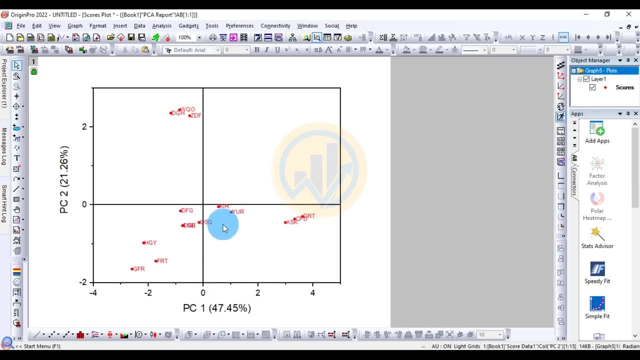 for the scar plot. okay, the next one for the scar plot. okay, the next one for the scar plot for the locations. this is location for the for the locations. this is location for the for the locations. this is location for the PC. one on the PC to further scatter. 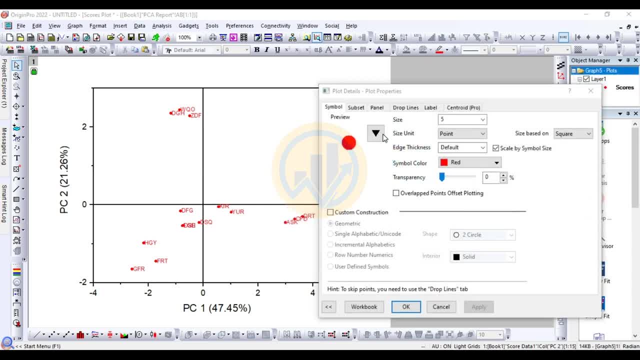 PC. one on the PC to further scatter PC. one on the PC to further scatter plot type. the double click for the plot type. the double click for the plot type. the double click for the locations that change for the symbols. locations that change for the symbols. locations that change for the symbols. okay, change color. change color anyone. 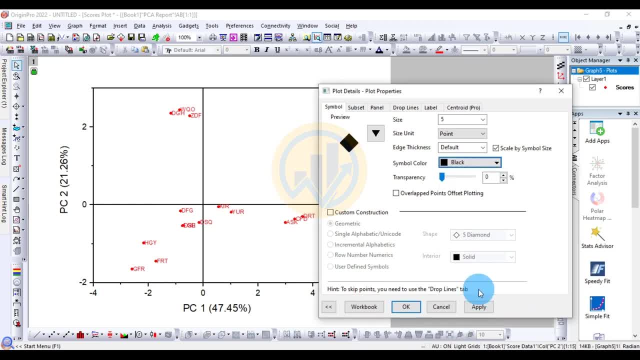 okay, change color, change color anyone. okay, change color, change color anyone. choose the red or black. okay, change the. choose the red or black. okay, change the. choose the red or black. okay, change the black black. okay, change the black or choose the bi-point color. also the change the. 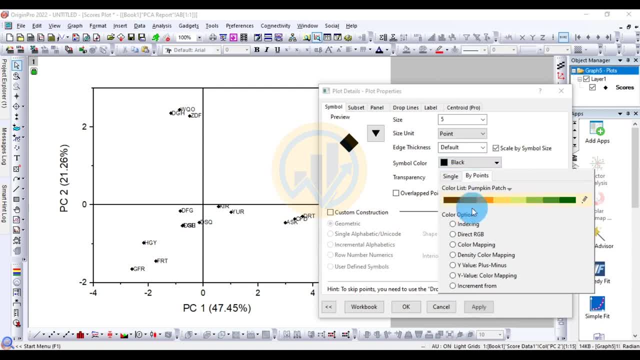 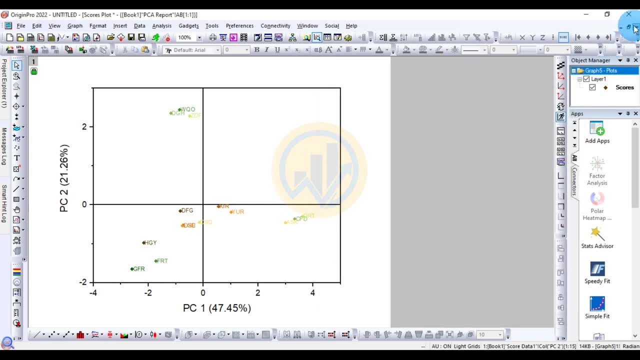 or choose the bi-point color, also the. change the. or choose the bi-point color, also the. change the multiple colors locations, then multiple colors locations, then multiple colors locations, then okay. the change colors, then okay, the okay. the change colors, then okay, the okay, the change colors, then okay. the next one for the, the bipolar part of the. 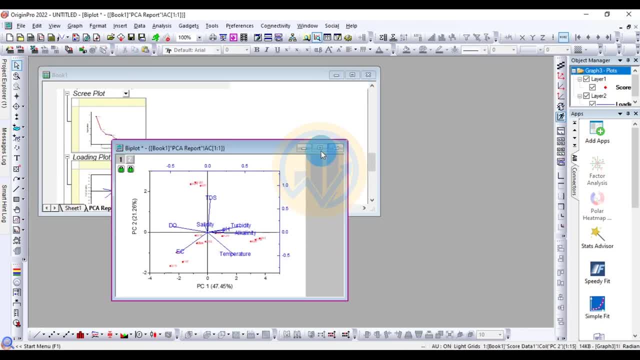 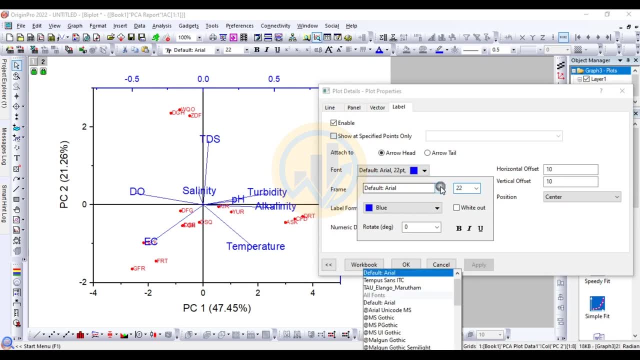 next one for the. the bipolar part of the next one for the: the bipolar part of the location under the water parameters: okay. location under the water parameters: okay. location under the water parameters: okay. the change for the water parameter: the. the change for the water parameter, the. the change for the water parameter, the change, the font. 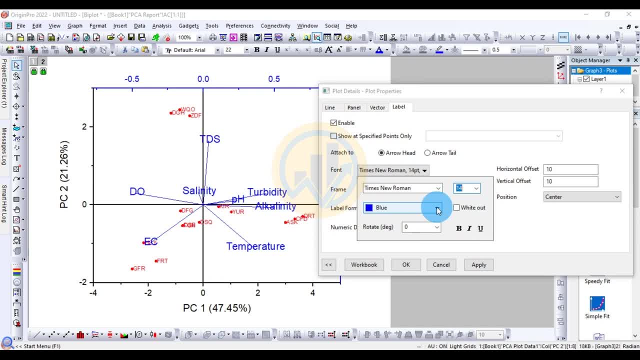 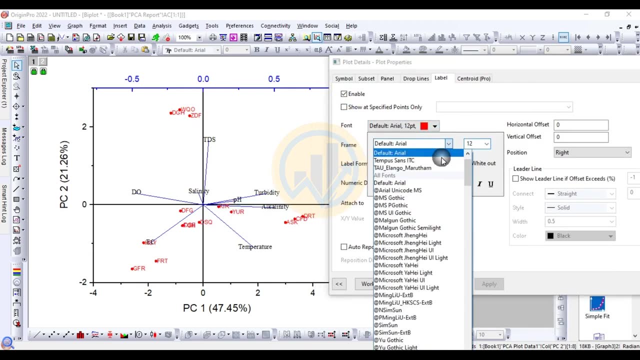 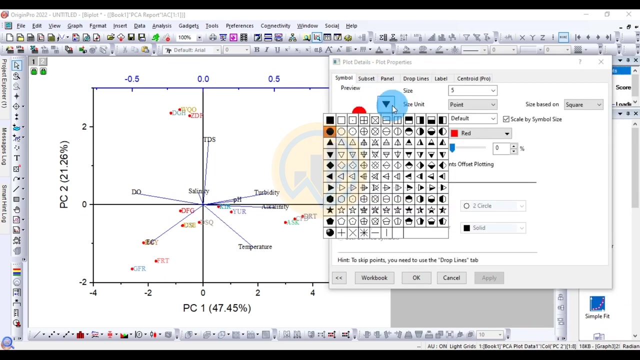 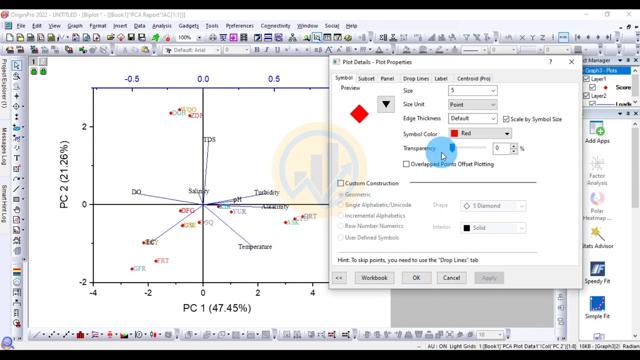 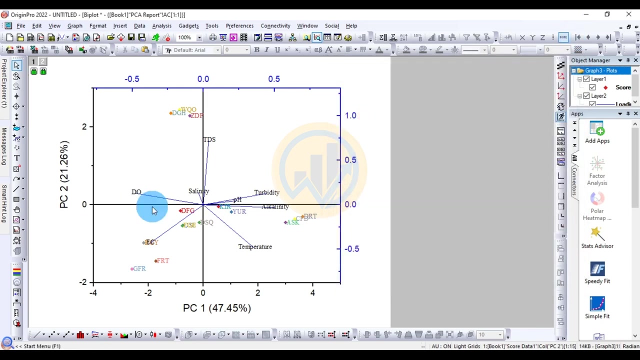 change the font. change the font: ok. the next one W for the locations: ok. the next one W for the locations: ok. the next one W for the locations. in the. change the location colors. change for the simple diamond: okay. change auto color or change any single color. then click the okay. this is for the scatter plot, where the principal compound analyzes. 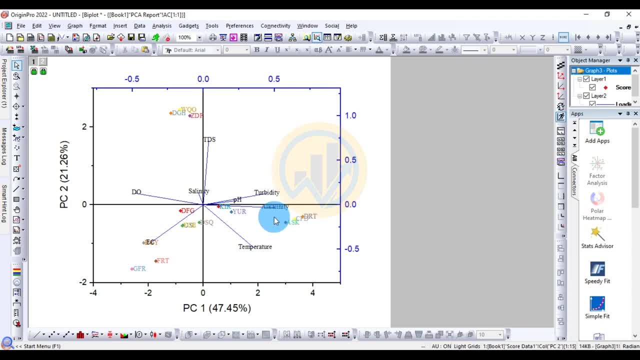 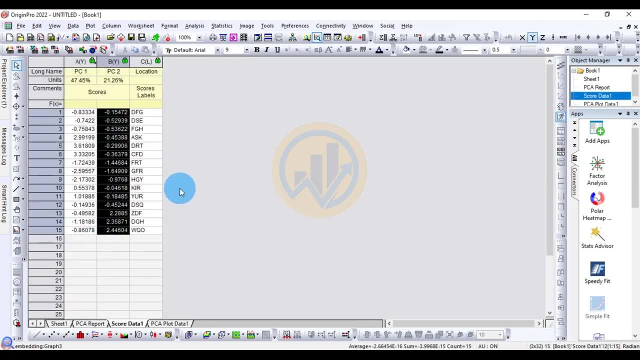 the PC 1 and the PC 2, the positive value and percent value. also the mention, the table value, the next one for the, the score data and the score data, the PC 1, PC 2, under location, so the score data, the mostly present out of the data, and forty seven point forty five percentage in the PC 1. on 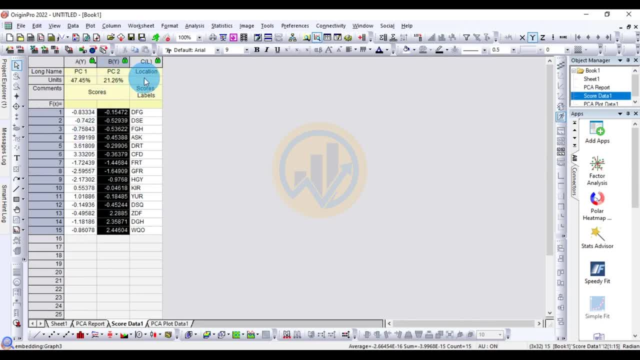 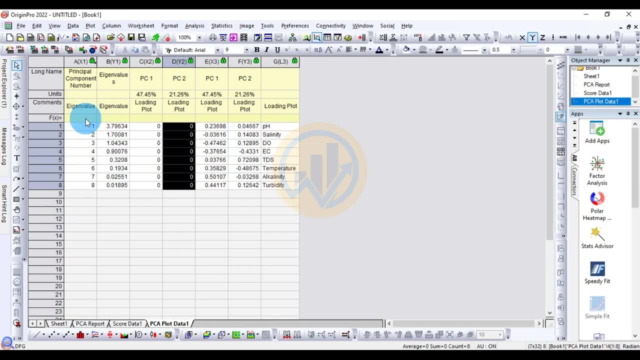 PC 2, is it 21.26? the location score label. mention the value. the next one for the pc plot data one. this is the principal component as eigen value for the eight value. then mention the eight values under the pc1 and pc2. for the value 47145, loading plots under the 21.26 percent. 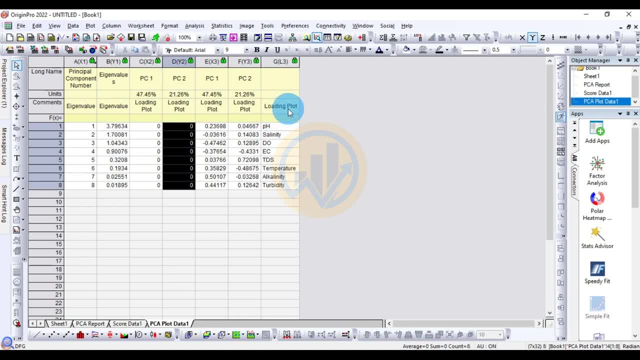 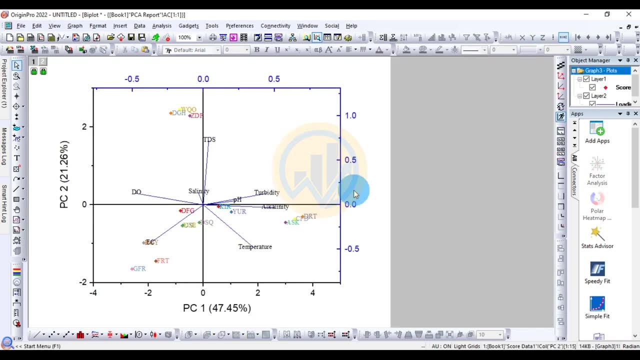 also the loading plot. the value mentioned is the location loading a plot. the label mentioned about the ph, salinity, doe, cdds, temperature, alkalinity under terminity, this is for the principal compound analysis in the origin pro software. thank you for watching this video.